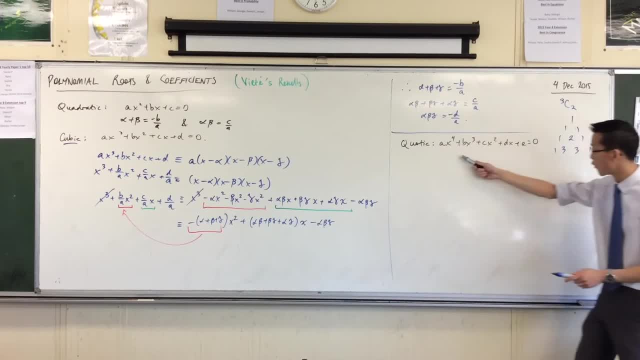 So here's a general quartic. right, it has 5 coefficients in here. it should have how many roots? 5, right? So I used alpha, beta and gamma before. now I'm going to add back in. I've showed you this before. I'm going to add in delta. sorry, 4, I mean I was counting 4, and I said 5, anyway. 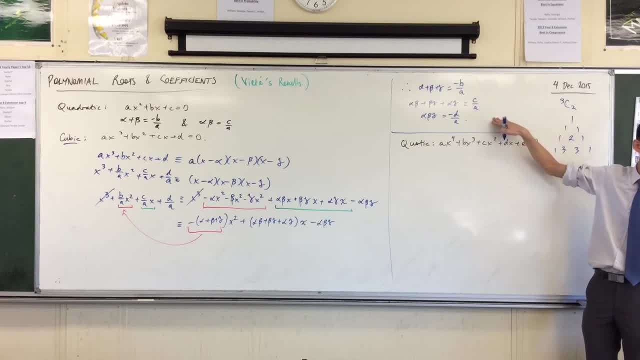 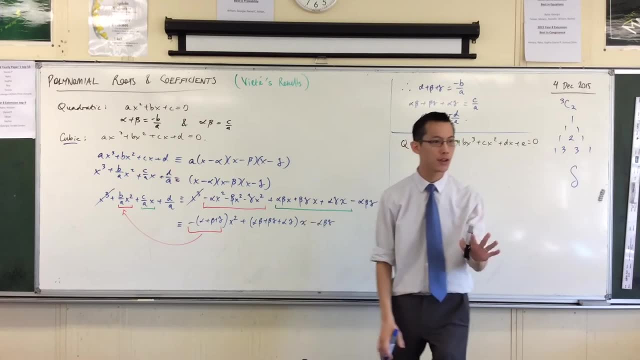 So I've got 4 roots right. So what are my relationships going to be When I add them all up? think about it this way: I'm going to write this first step here, but I'm not going to do any of the expansion. I'll see if you can follow this. 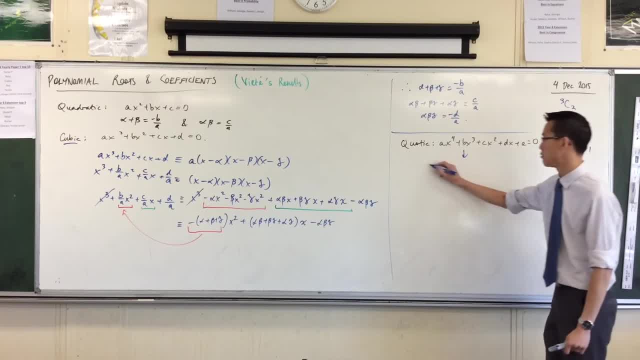 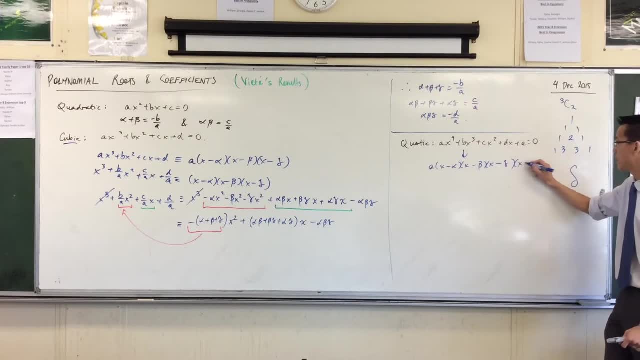 This is the argument, right? If this thing should be equivalent to a times, let's put the 4 roots in here. so this is the 4 linear factors that I should be getting delta if there are 4 roots. again, think about, for instance, how am I going to get an alpha at the end here, right? 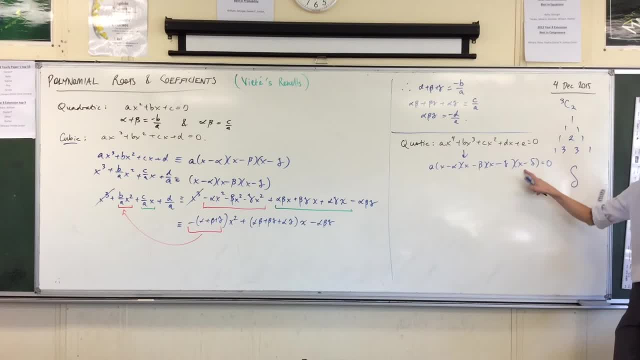 Well, if I get that alpha, it's going to multiply by x, x, x, right? So you're going to get an x cubed term. so I'm comparing to this guy. right To get a beta. there's a beta there. 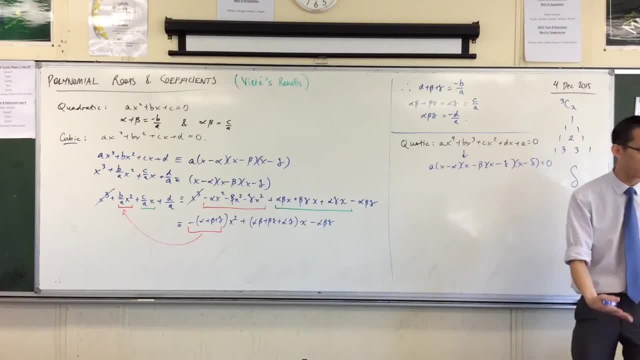 And again you're going to have to choose the x here and the x here and the x here. Again, you're getting an x cubed. Again, you're comparing to this b coefficient, right? Whatever, the second one was okay. 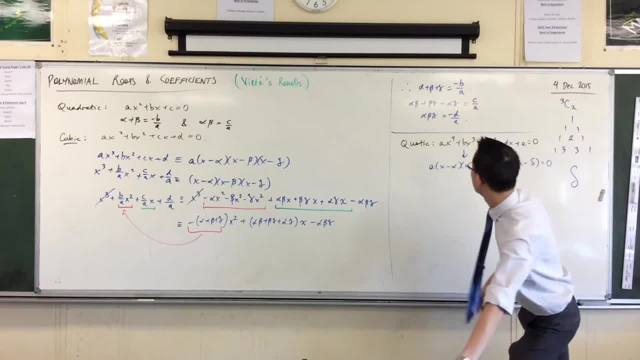 So therefore, without any actual algebraic expansion, let's write out the roots and coefficients, those results for a coin. It's not hard to follow the pattern. You do the sum one at a time and it's still amazingly minus b on a. 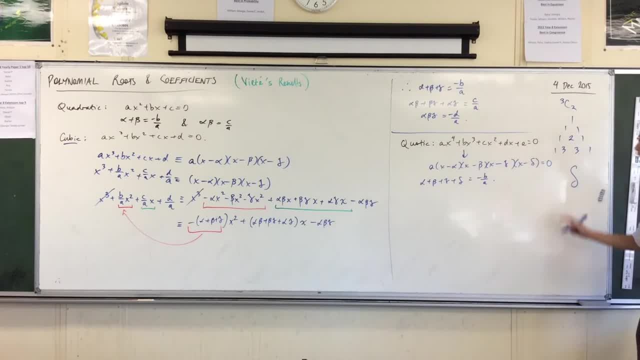 You do the sum two at a time. now this is a bit trickier. okay, We're going down to one. four, six, four one. so this is the next row of Pascal's triangle. right, I've already got this. this is the four that's here. that's four c one. now I'm doing four c two, so I should expect six terms. 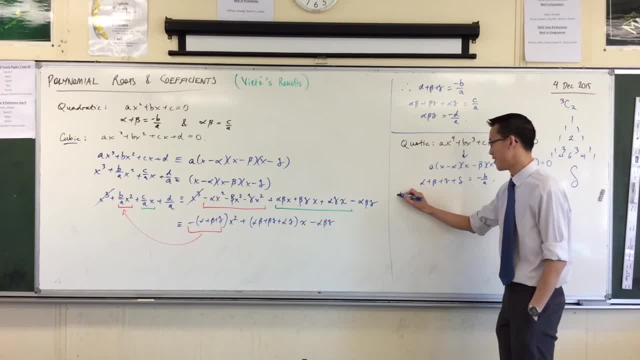 That's how I know I wouldn't have missed any. okay, Help me out. Alpha beta, I do. I tend to do all the alphas first, so I'll go: alpha beta, alpha gamma, alpha delta, okay. 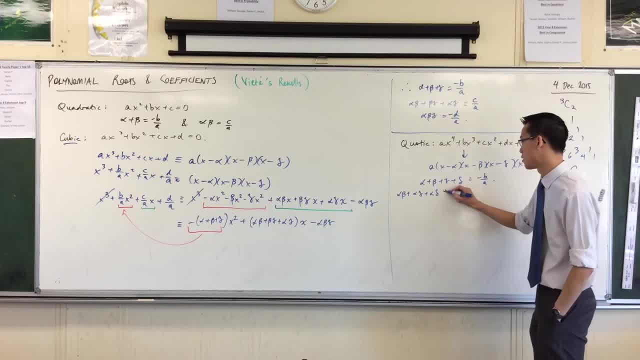 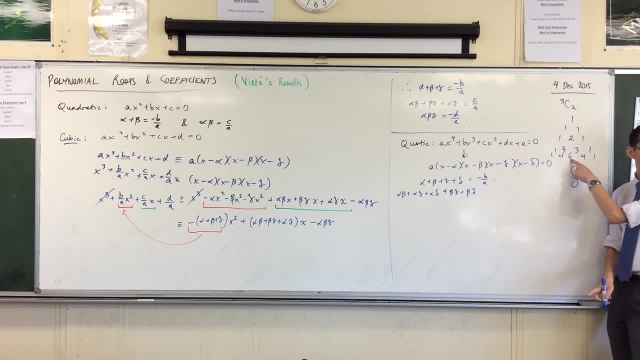 Then I do all the betas next. I've already done alpha beta, so I'll do beta, gamma and beta delta. now look, I've got five. Pascal's triangle tells me I'm only missing one more, which is the gamma delta. the very last pair, right? 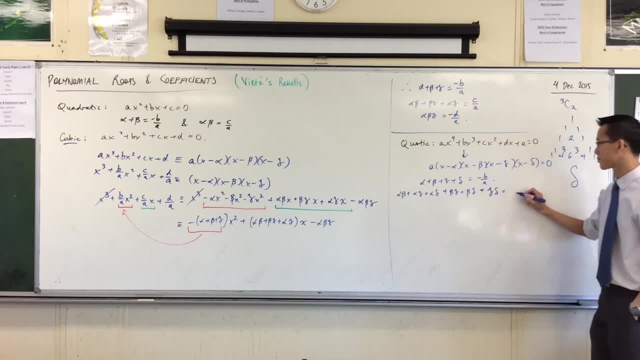 Another way: gamma delta. another way that I can know is: you look at how many times you've used each of the roots. okay, How many times have I used alpha? namely One, two, three times. right, You can only use it three times because it only has three other things to pair up with. 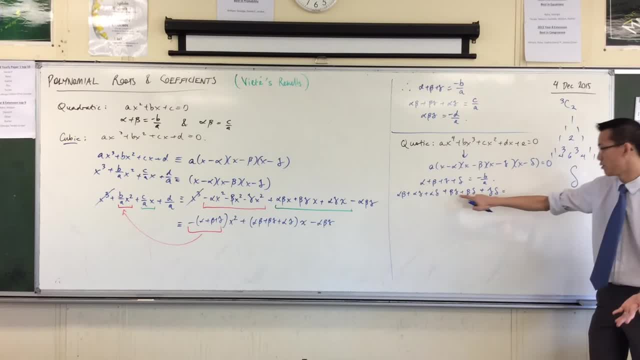 How many times have you used beta? One, two, three times, because there are only three other things it can pair up with. How many times have you used gamma? Uh, hold on One, two, three and you can see. I don't need to do delta for you, do you? I've got three as well, okay. 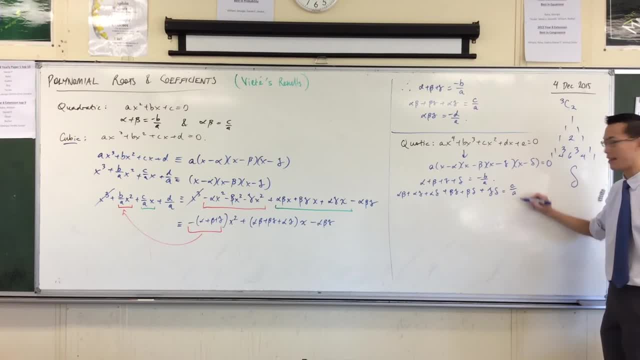 Now again, the coefficients are going to go to the next one and the sign is going to alternate. Now we do them three at a time. how many terms am I going to expect? Four of them, because I've gone to the next one in Pascal's triangle. 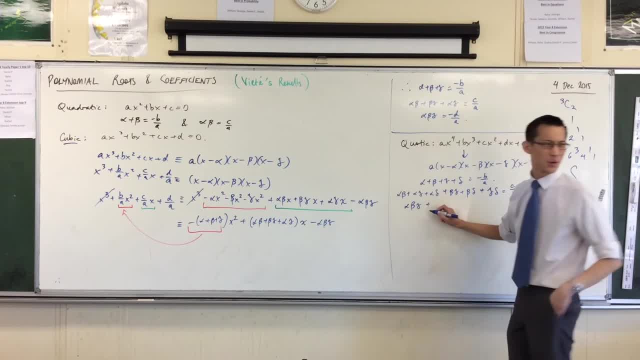 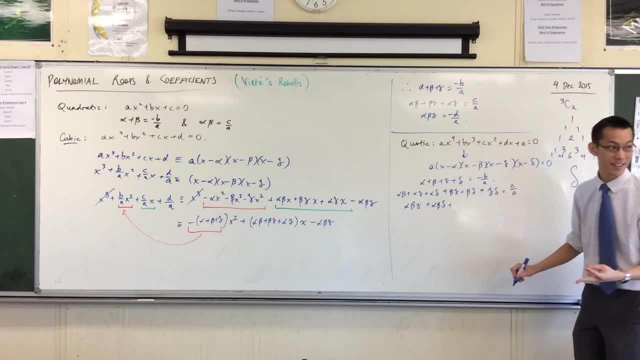 So I'm going to go- this is a bit harder- Alpha, beta, gamma. I do all the alphas first. yeah, Alpha, beta, delta. okay, I'm only missing two more. Someone help me out. I can do beta, gamma, delta, and I'm missing one last one. 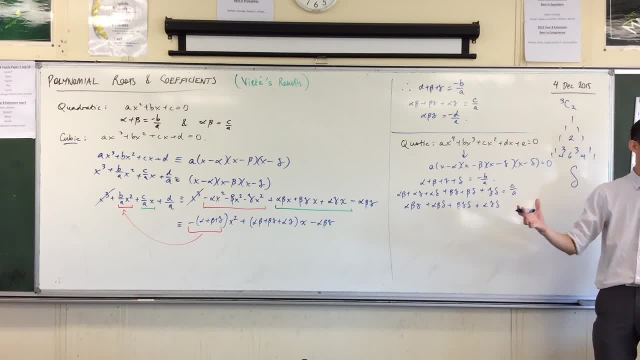 Alpha gamma delta- perfect Again, I can check how many times have I used alpha One, two, three times. How many times have I used beta One, two, three times? Do you need me to do this? 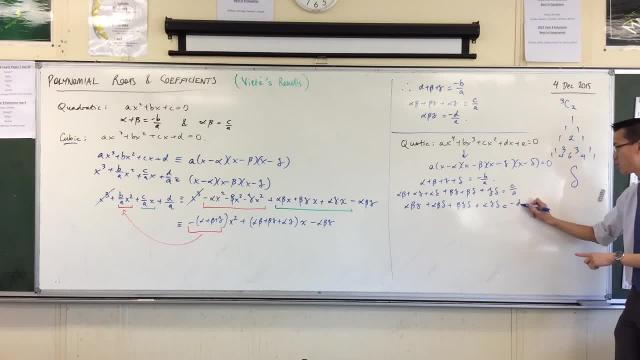 Like you can see right, And the sign alternates and you go to the next coefficient. Mercifully, the last one is easy to do: The sum- oops, sorry, the sum- four at a time: alpha, beta, gamma, delta- and it's, the sign alternates and you go to the next coefficient. 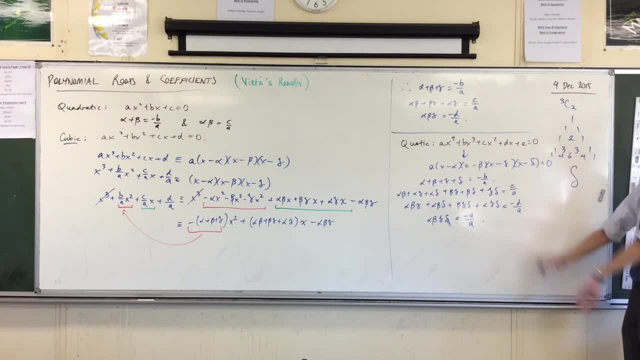 Done. There are the results for the Quantic. okay, Can we use a different like? what's it called? You can use any. you can use any. You can use any letter you like. However, this is the letter that gets traditionally used and, like I mean, I think it's worth learning because you will see it. 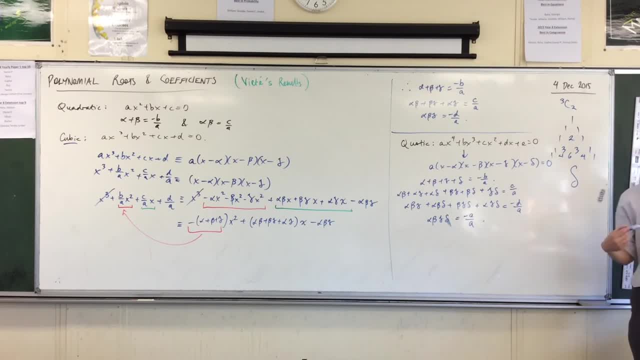 I don't like the delta. Yeah, you don't have to use delta. yeah, When you're multiplying four negative roots together, shouldn't you get a positive number instead of negative? You're talking about this one. hold on this one here. 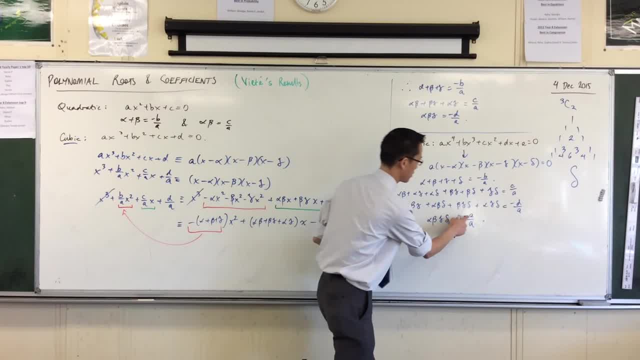 Yeah, it's meant to be positive. Oh yeah, so it's E on it. Oh yeah, of course it is. yeah, My sign alternated. Okay, great, Any was that is that? it Is that the basic, yet.